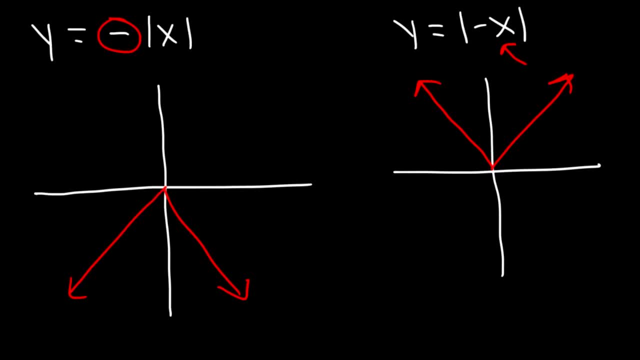 on the outside will. Now, what are the domain and range of these two functions? The domain represents all of the values. The domain represents all of the possible x values. As you can see, x can be anything. The lowest x value all the way to the left is negative infinity and the highest is infinity. 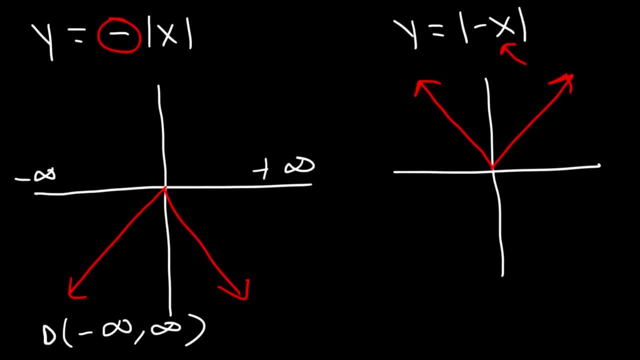 So it's all real numbers for the domain. You can plug in any value into x. Now what about the range? The domain for the other one is the same, by the way, It's negative infinity to infinity. That's going to be true for all absolute value functions if there's no fractions, no radicals. 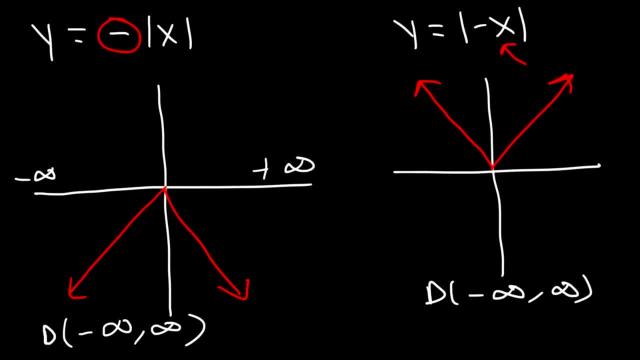 no logarithmic equations, It's going to be all real numbers. Now, as for the range, what's the lowest y value that we see in the graph on the left? Notice that it goes down towards negative infinity. and the highest y value is 0.. 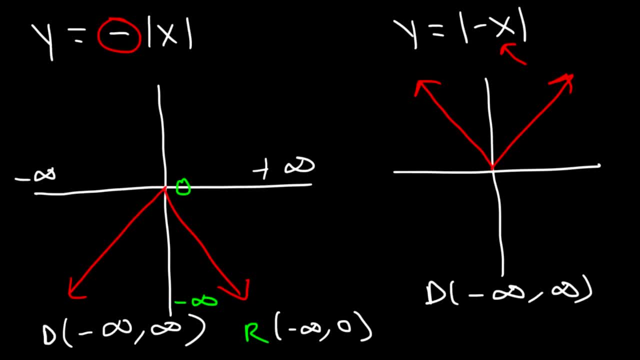 So the range is from negative infinity to 0.. Now for the graph on the right. the lowest y value is 0, the highest is infinity. So the range is from 0 to infinity, 0 to infinity, 0 to infinity. 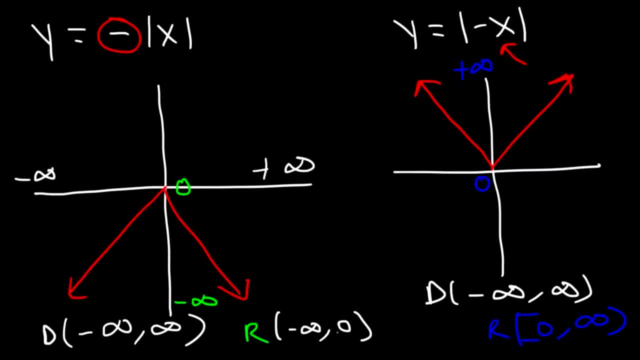 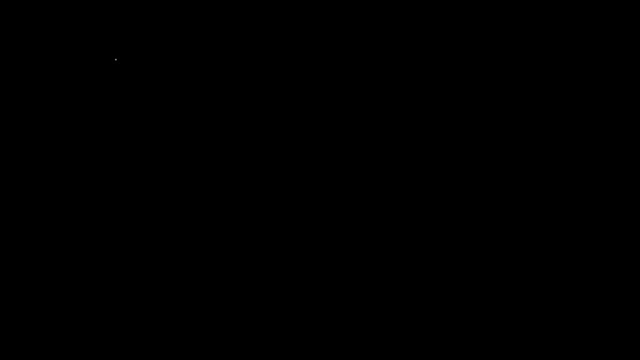 0 is included, so we need to use a bracket instead of a parenthesis. Now, what about graphing an equation that looks like this: This graph is going to shift two units to the left, and so it's going to open upward because there's a positive outside of the absolute value function. 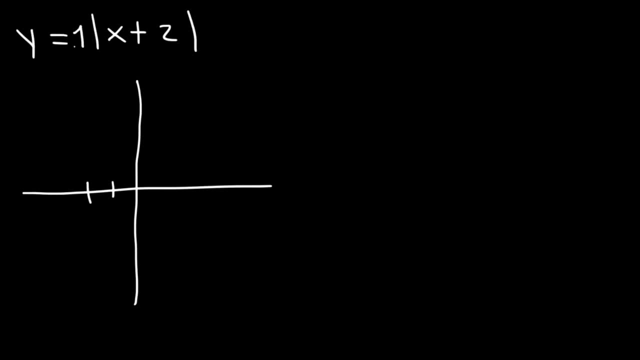 Now, if you want to plot points, you need to realize that the solution is going to be positive. You need to realize that the slope is 1.. So, once you plot the vertex, as you travel one unit to the right, go up one unit. 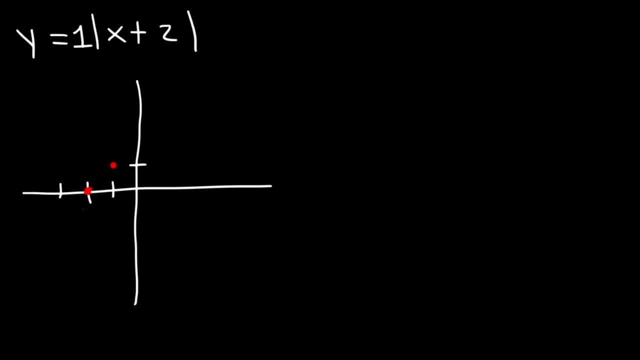 So that will take you to the point And as you travel one unit to the left, go up 1, because the slope is 1.. On the right side the slope is positive 1, but on the left side the slope is negative. 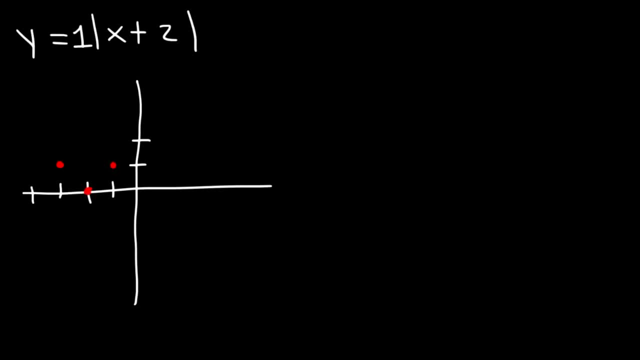 1.. And then, to find the next point, travel 1 to the right and up 1.. And the left side is just going to be a reflection of the right side. So the graph is going to look like this: If there was a 2 in front, the slope would be 2.. 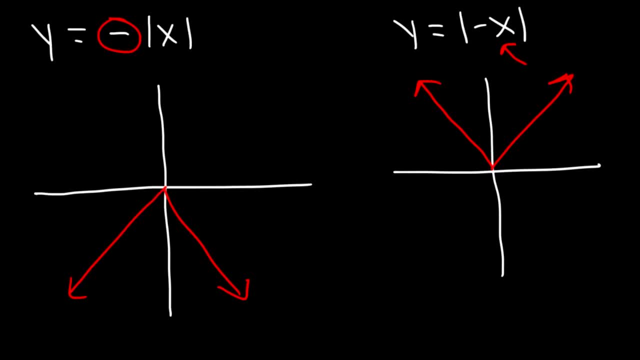 on the outside will. Now, what are the domain and range of these two functions? The domain represents all of the points. The domain represents all of the possible x values. As you can see, x can be anything. The lowest x value all the way to the left is negative infinity and the highest is infinity. 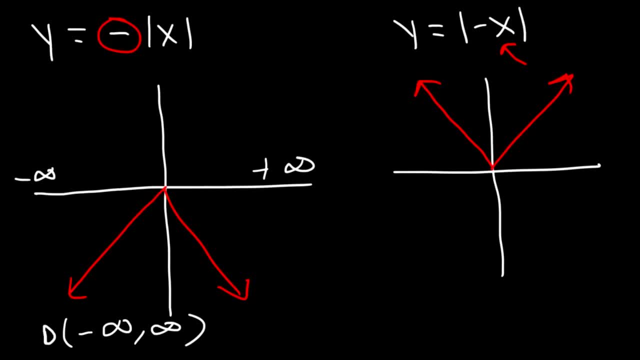 So it's all real numbers for the domain. You can plug in any value into x. Now what about the range? The domain for the other one is the same, by the way, It's negative infinity to infinity. That's going to be true for all absolute value functions if there's no fractions, no radicals. 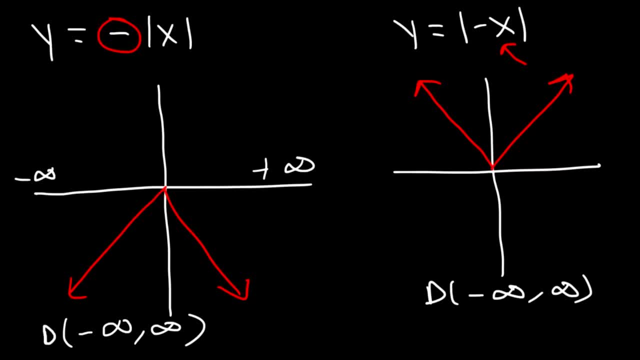 no logarithmic equations, It's going to be all real numbers. Now, as for the range, what's the lowest y value that we see in the graph on the left? Notice that it goes down towards negative infinity. and the highest y value is 0.. 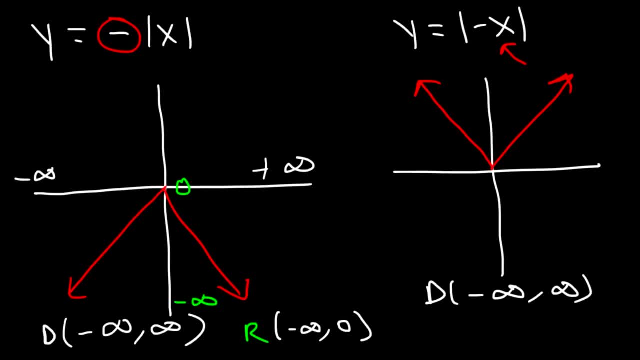 So the range is from negative infinity to 0.. Now for the graph on the right. the lowest y value is 0, the highest is infinity, So the range is from 0 to infinity, And 0 is the highest value, So the range is from 0 to infinity. 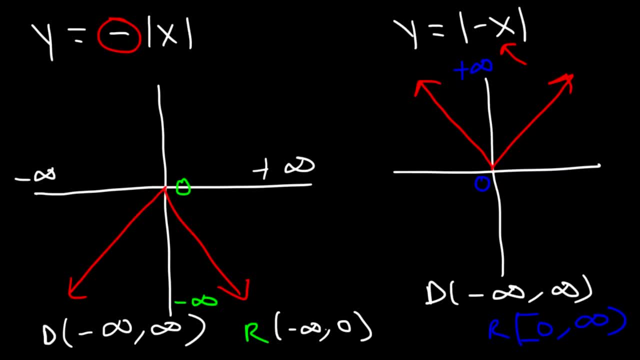 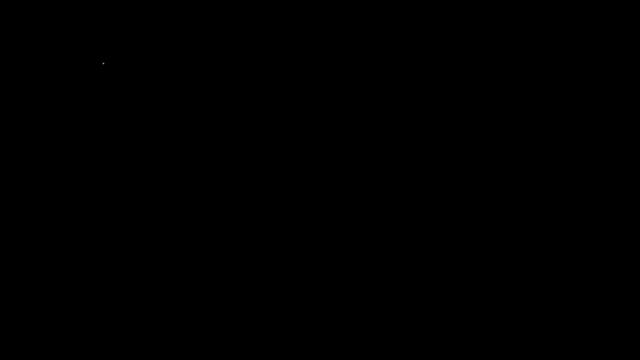 And 0 is included, so we need to use a bracket instead of a parenthesis. Now, what about graphing an equation that looks like this: This graph is going to shift two units to the left, and so it's going to open upward because there's a positive outside of the absolute value function. 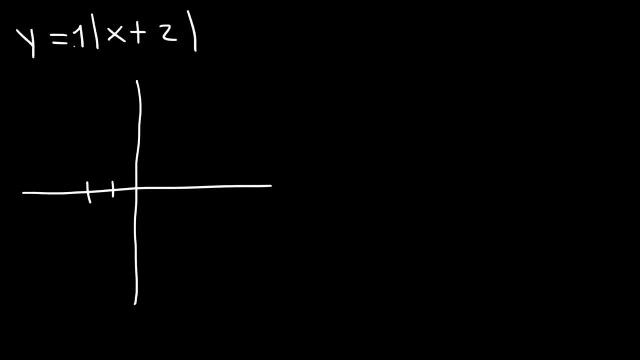 Now, if you want to plot points, you need to realize that the slope is 1.. So, once you plot the vertex, as you travel one unit to the right, go up one unit, So that will take you to the point. And as you travel one unit to the left, go up one, because the slope is 1.. 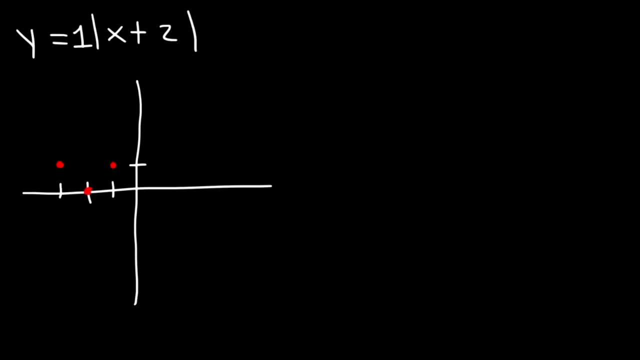 On the right side, the slope is positive 1, but on the left side, the slope is negative 1.. And then, to find the next point, travel 1 to the right and up 1.. And the left side is just going to be a reflection of the right side. 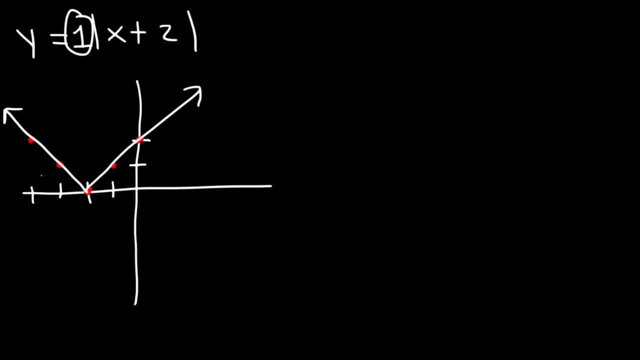 So the graph is going to look like this: If there was a 2 in front, the slope would be 2.. The graph would be more steeper, so to speak. It would be narrow and not as wide. Now, what about the graph for this one x minus 3?? 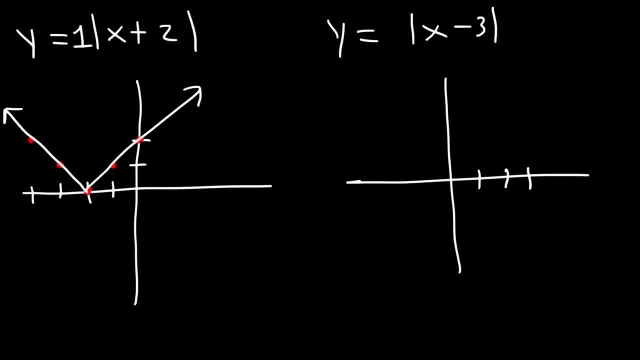 This one is going to shift 3 units to the left, And the left side is just going to be a reflection of the right side, And it's still going to open in the upward direction with a slope of 1.. Now, what about the absolute value of x plus 2, and also negative absolute value of x minus? 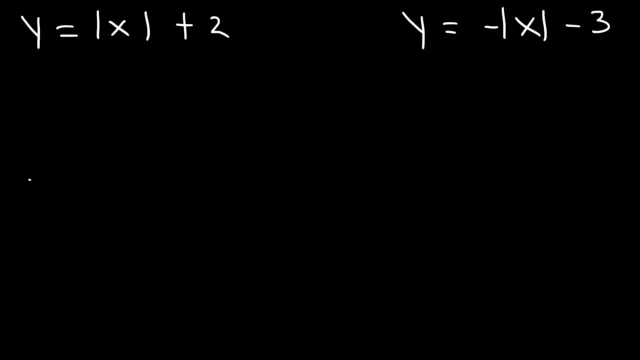 3? What's going to happen to the graph? In the first example, it's going to shift up 2 units and, because we have a plus sign in front, it's going to open up In the upward direction. For the second example, it's going to shift down 3 units. 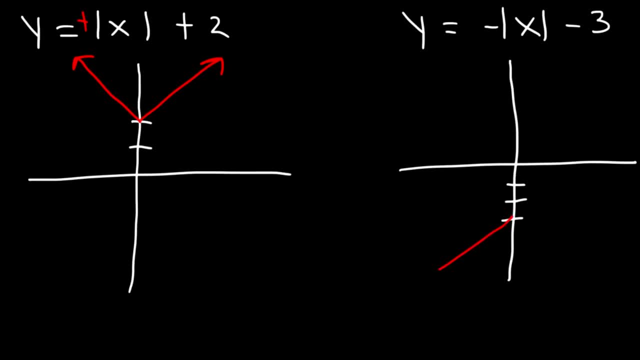 That's a vertical shift. Left and right represents a horizontal shift And it's going to open downward due to the negative sign. Now, what are the range for the graph for each of these? Let's start with the first one. what's the range? 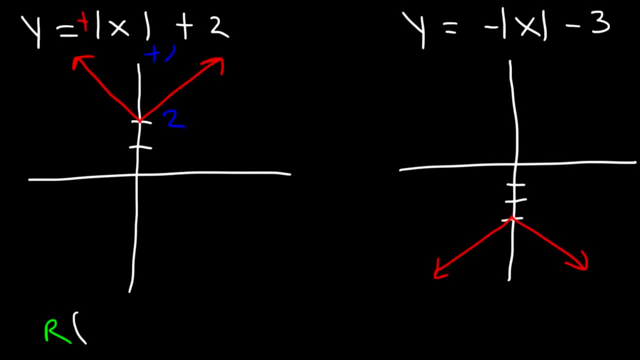 Notice that the lowest y value is 2.. The highest is infinity. So the range is going to be from 1 to the left, 2 to infinity, And 2 is included. Now for the one on the right, the lowest y value is negative infinity. 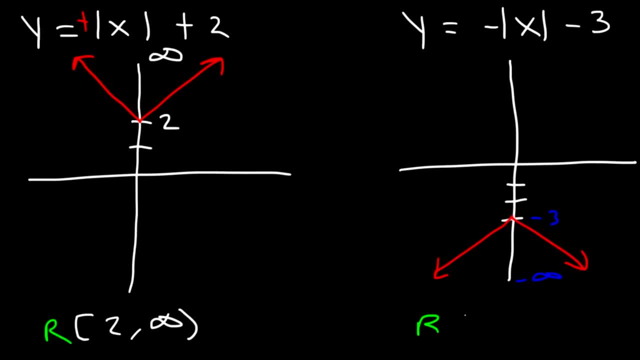 The highest is negative 3.. And negative 3 is included, So the range is from negative infinity to negative 3.. You start from the low y value and you stop at the highest y value, And there's no breaks in between. 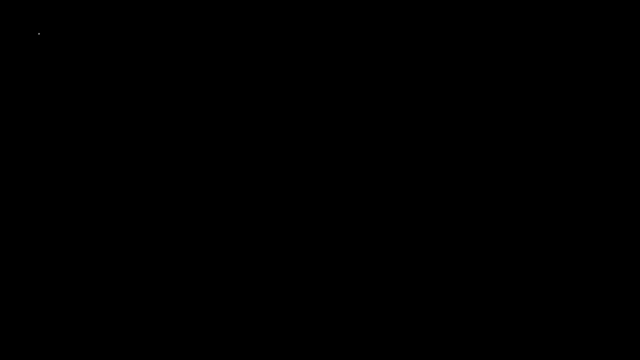 So that's the first one. Next Now, what you see right here are lots of options. So what if we have a combination? Let's say this graph: It's going to shift 2 units to the right and up 3 units. 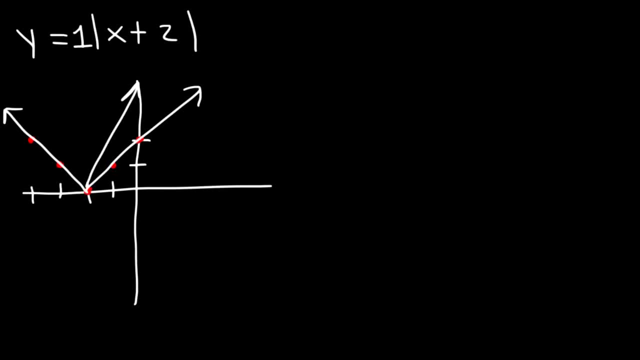 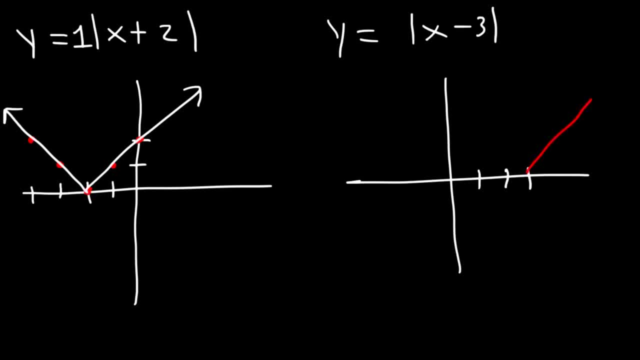 So now this is going to shift 3 units to the right And it's still going to open in the upward direction with a slope of 1.. Now what about the absolute value of x plus 2? And also negative absolute value of x minus 3?? 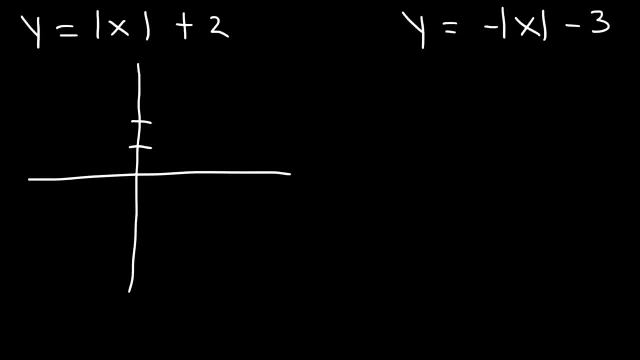 What's going to happen to the graph? In the first example, it's going to shift up 2 units And, because we have a plus sign in front front, It's going to open in the upward direction. For the second example, it's going to shift down. 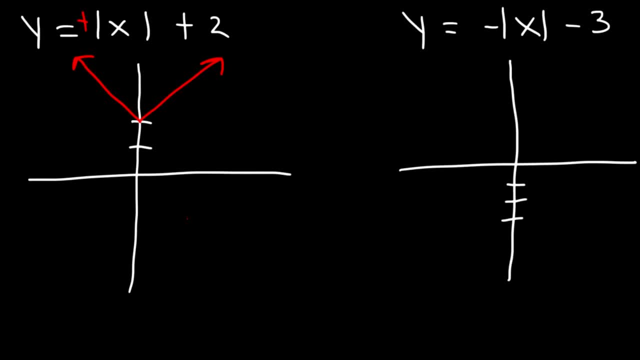 three units. That's a vertical shift. Left and right represents a horizontal shift and it's going to open downward due to the negative sign. Now, what are the range for the graph for each of these? Let's start with the first one. What's the range? 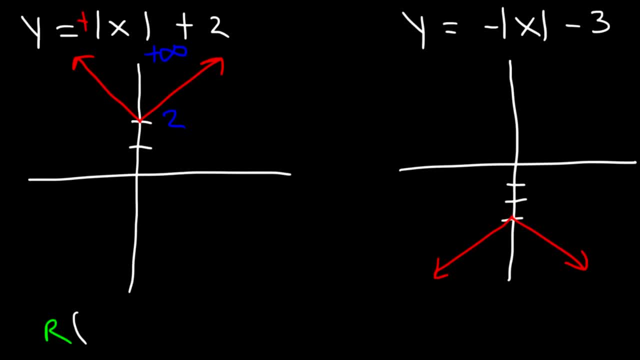 Notice that the lowest y value is 2.. The highest is infinity, So the range is going to be from 2 to infinity, and 2 is included. Now for the one on the right: the lowest y value is negative infinity. The highest is negative 3, and negative 3 is included, So the range is from: 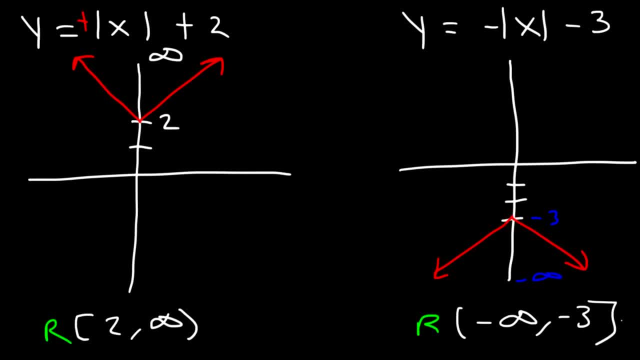 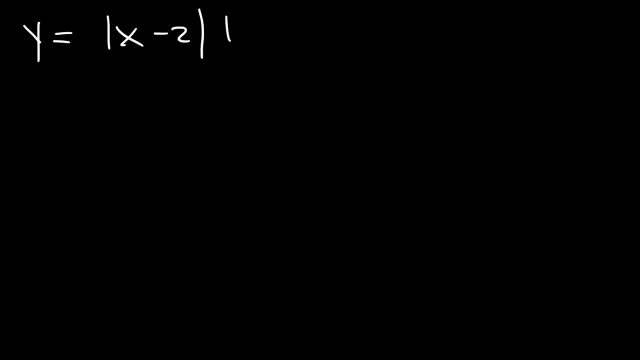 negative infinity to negative 3. You start from the low y value and you stop at the highest y value and there's no breaks in between. So what if we have a combination of transformations? Let's say this graph: So it's going to shift two units to the right and up three units. So 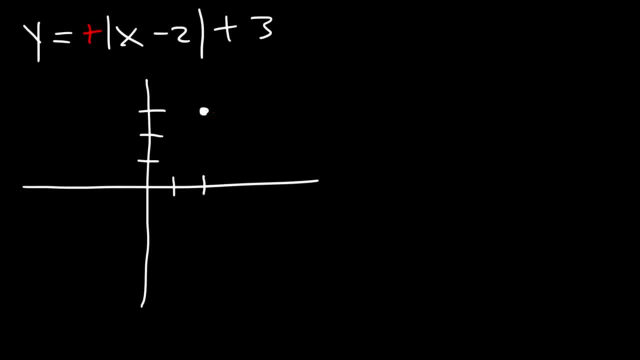 here's the vertex, and it's going to open upward, with a slope of 1 to the right and with a slope of negative 1 to the left. By the way, for those of you who prefer to use tables, here's what you. 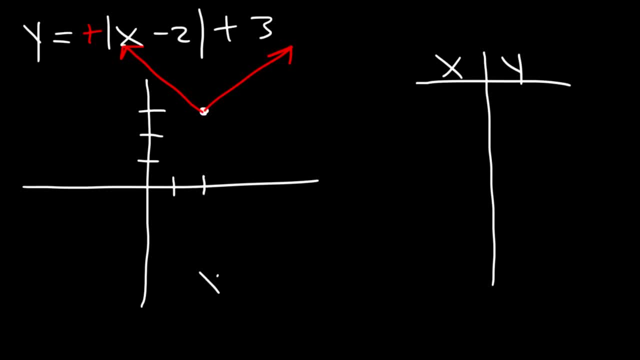 want to do. If you set the y value to negative 1, you're going to have a slope of 1 to the right, and if you set the inside part equal to 0, this will give you the x-coordinate of the vertex. 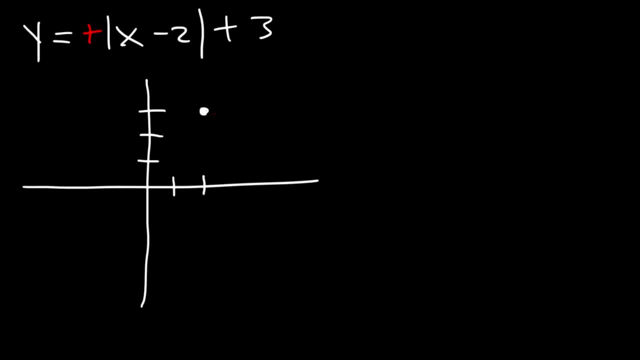 So here's the vertex. For those of you who prefer to use tables, here's what you'll want: use inside part equal to zero. This will give you the x coordinate of the vertex, which is two. After that, you want to make that your center point. Choose two points to the right of two. 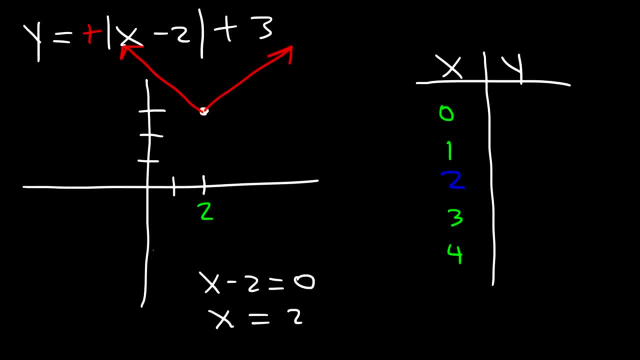 and two points to the left and find the y values at those points. When you plug in two, y is going to be three. When you plug in three, the absolute value of three minus two is one plus three. That's going to be four. If you plug in one, it's going to be the same thing. 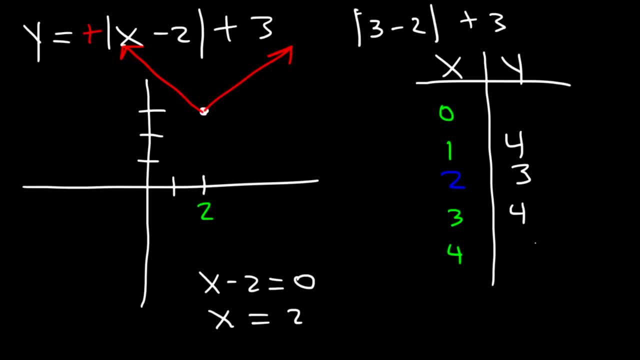 If you plug in four, four minus two is two plus three is five. If you plug in zero, you're going to get the same thing, And once you plot it, you're going to get a graph that looks like this: The domain for that graph is all real numbers, but the range the lowest, y. 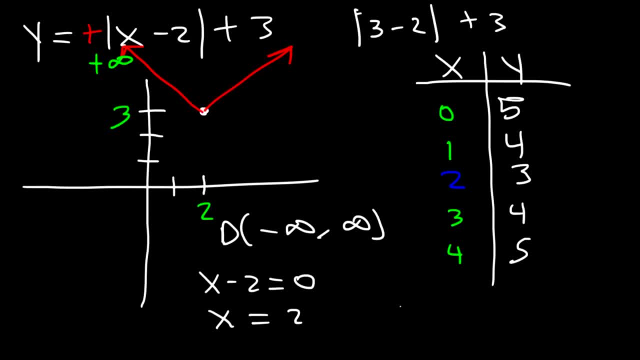 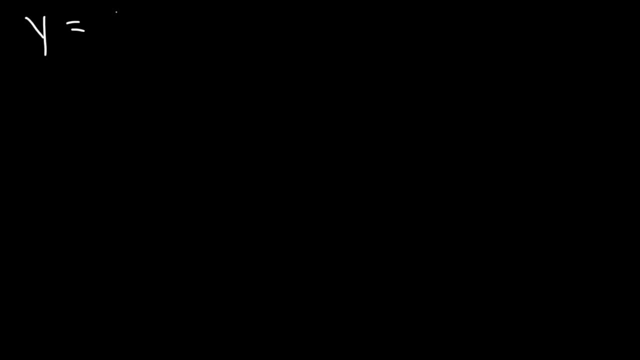 value is three. the highest is infinity. So the range is going to be three to infinity. Try this, Try this: one Four minus the absolute value of x plus one. So the graph is going to shift one unit to the left and it's going to shift up four units. 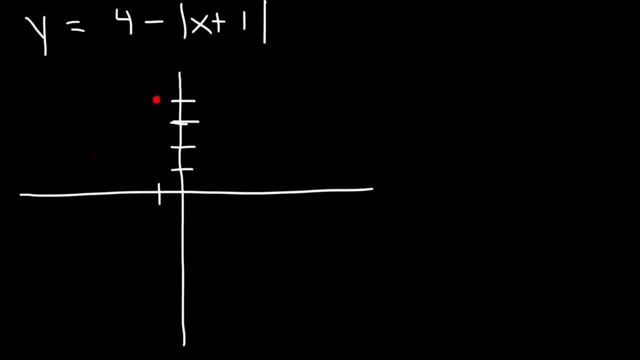 So the vertex is at the point negative one comma four, And the slope, the number in front of the absolute value function, is one, And because there's a negative sign in front of it, we know it's going to open in the downward direction. But let's plot points though. 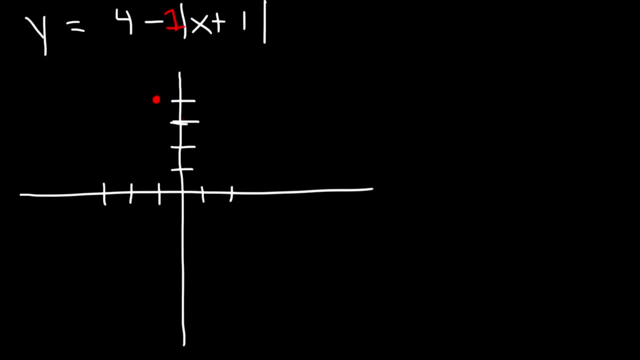 To get the next point, as you travel one unit to the right, you need to go down one Same thing. one to the left, go down one, And then one to the right. go down one again and just repeat the process. 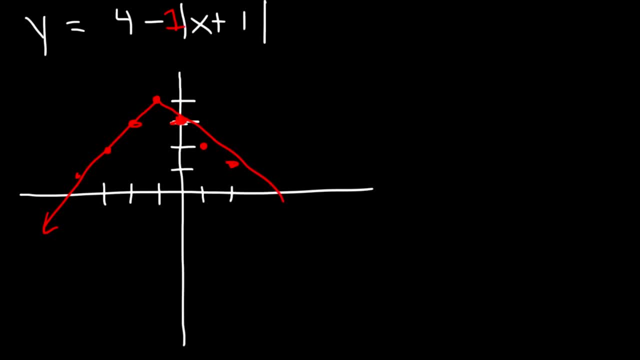 And so this is going to be a rough sketch of the graph And I missed all the points there. So that's how you can graph it If you want to draw a more accurate sketch using points- And, as we can see, the range is from negative infinity to four- 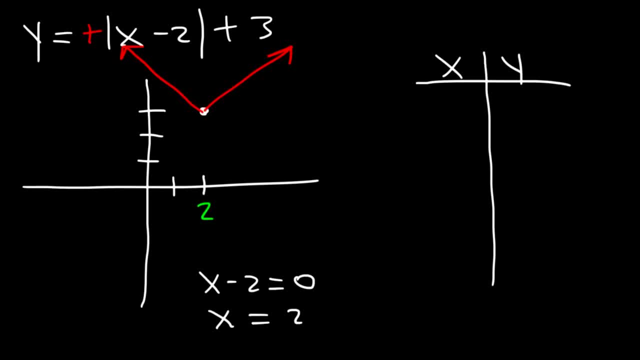 which is 2.. After that you want to make that your center point. Choose two points to the right of 2, and two points to the left, and find the y values at those points. When you plug in 2, y is going to be 3.. When you plug in 3,, the absolute value of 3 minus 2 is 1 plus 3,. 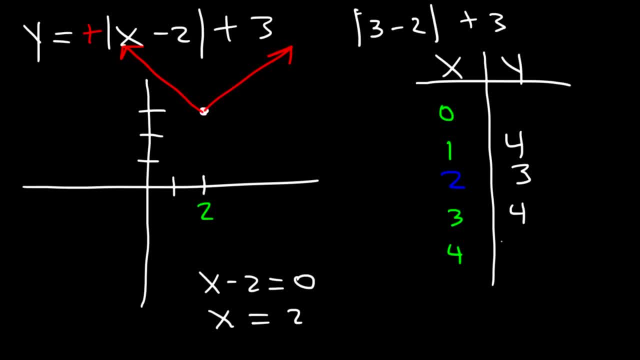 that's going to be 4.. If you plug in 1,, it's going to be the same thing. If you plug in 4,, 4 minus 2 is 2 plus 3 is 5.. If you plug in 0,: 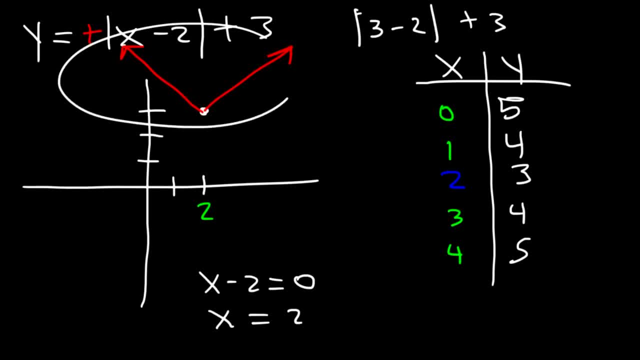 you're going to get the same thing And once you plot it, you're going to get a graph that looks like this: The domain for that graph is all real numbers, but the range, the lowest y value, is 3,, the highest is infinity. So the range is going to be 3 to infinity. Try this one: 4 minus the. 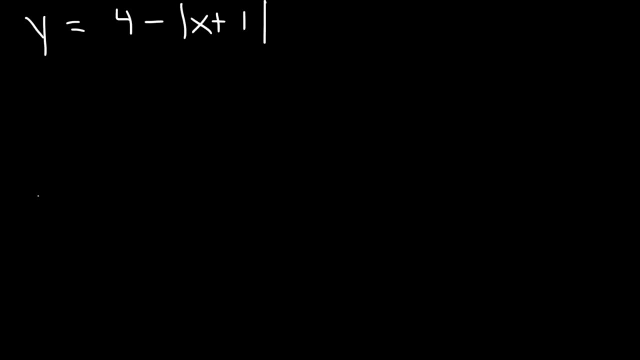 absolute value of x plus 1.. So the graph is going to shift 1 unit to the left and it's going to shift up 4 units. So the vertex is at the point negative 1 comma 4.. And the slope, the. 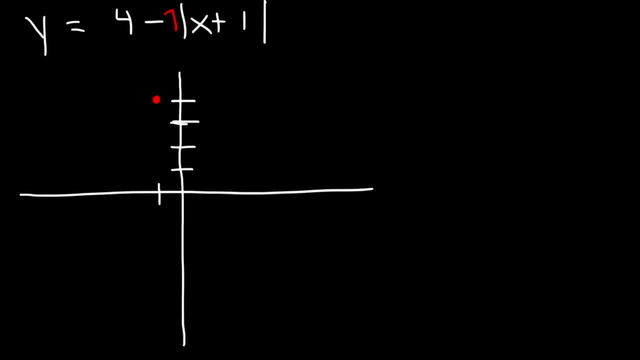 number in front of the absolute value function is 1.. And because there's a negative sign in front of it, we know it's going to open in a downward direction. But let's plot points To get the next point. as you travel 1 unit to the right, you need to go down 1.. Same thing. 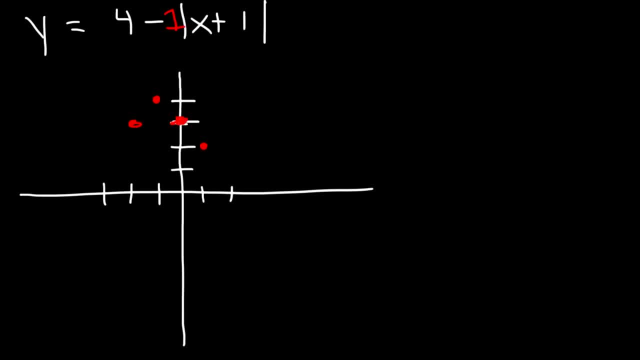 1 to the left, go down 1.. And then 1 to the right, go down 1 again and just repeat the process, And so this is going to be a rough sketch of the graph, And I missed all the points there. 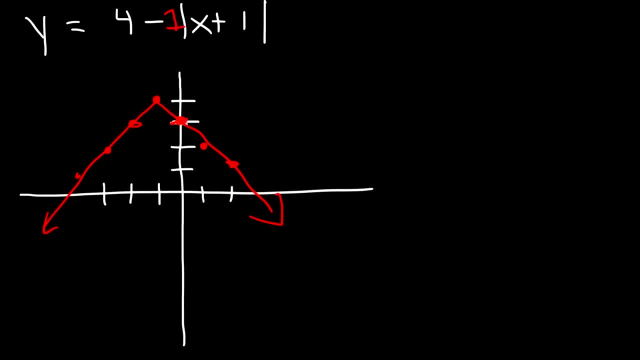 So that's how you can graph it if you want to draw a more accurate sketch, using point points And, as we can see, the range is from negative infinity to 4.. The highest y value is 4.. And don't forget to put brackets, because it includes 4.. Let's try one more example. 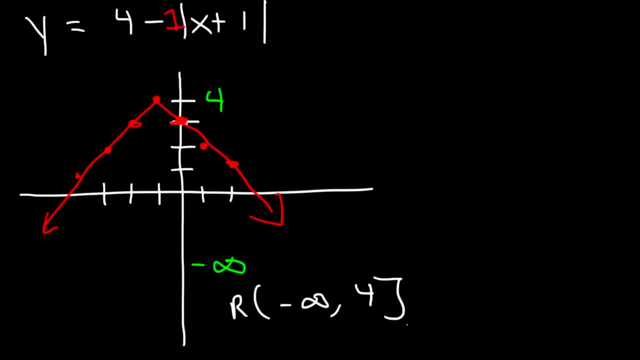 The highest y value is four, And don't forget to put brackets, because it includes four. Let's try one more example. So let's graph this one. So this time the slope is going to be two. The graph is going to shift one unit to the right. 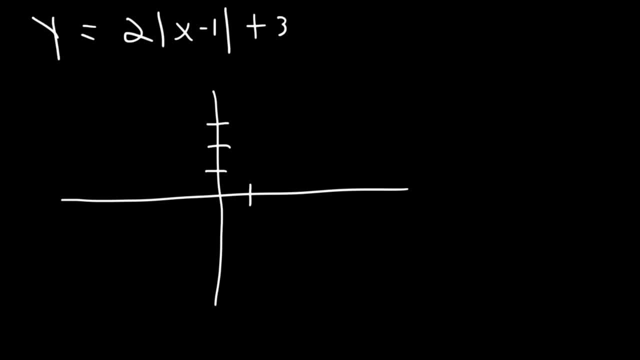 and it's going to shift up three units. So it starts at the point one. three As we travel: one to the right, we need to go up two units on the y-axis. So the next point is over here. One to the left, we need to go up two units. 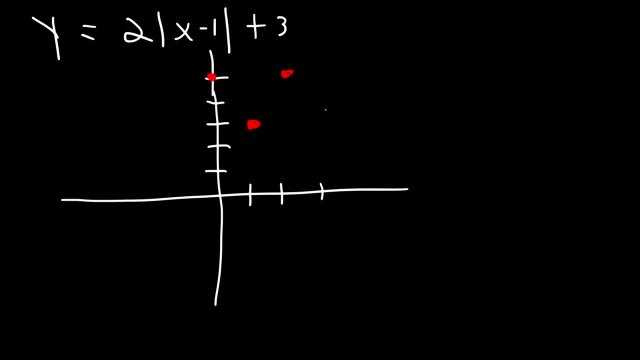 And as we travel, one more unit to the right and one to the left. we need to go up two more units, but I'm out of space, So I'm just going to have to go with this Because I'm out of space. let's do one more example. 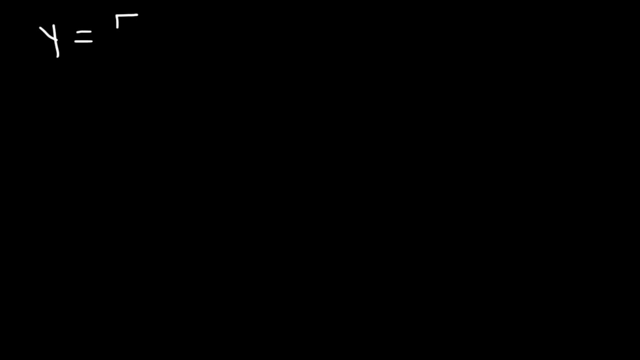 So let's say, if we have five minus three, x minus one- So I'm going to put this over here And draw a bigger graph this time- So as we travel one unit to the right, we need to go up five units. 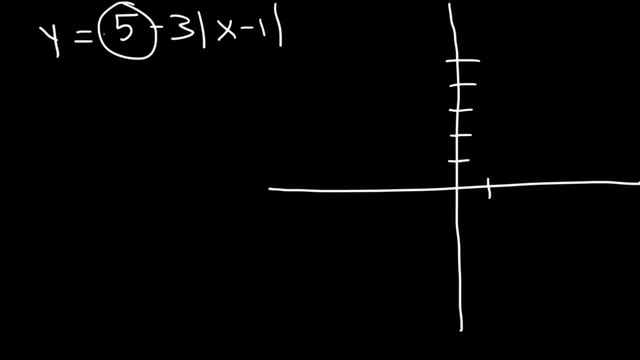 Based on this, it shifts one to the right horizontally and vertically up five units. So the first point is that 1 comma 5. now we have a slope of 3 and because it's negative, we know it's going to open downward. so as we travel, one unit to the right needs to go down three. 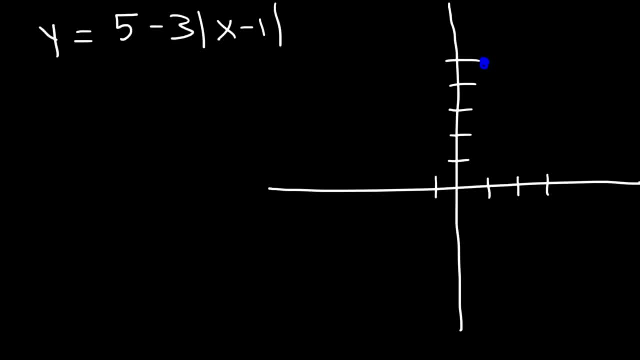 units 5 minus 3 is 2, so that will take us to the point 2, comma 2, and then, once to the left, we need to go down three units. so that's the point 0- 2, and then, if we go one more to the right, we need to go down three units. 2 minus 3 is 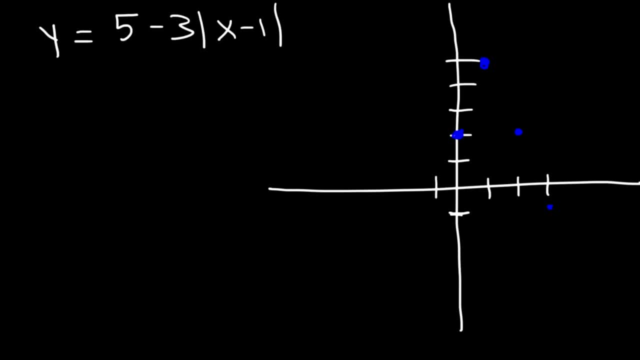 negative 1. so we'll get this point here and another one here, and if we go one more to the right and one to the left, we need to go down three more units. so the graph is going to look something like this. so now you know how to graph. absolute value functions.